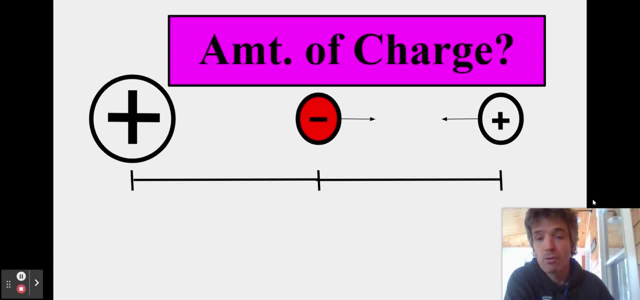 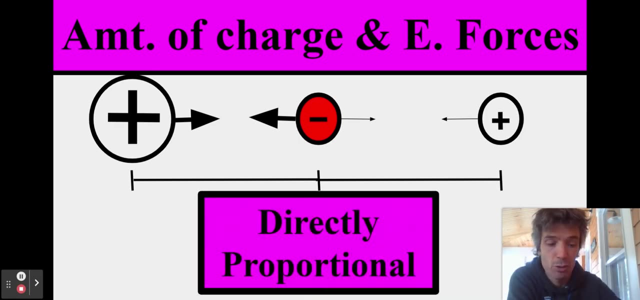 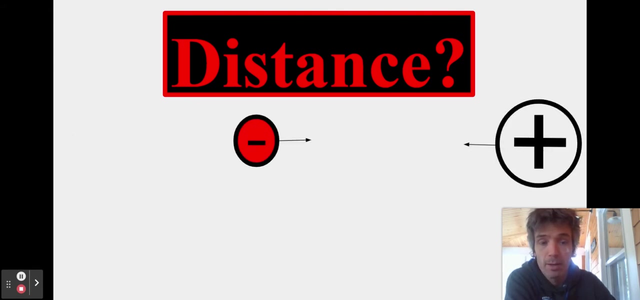 the other. Therefore, the one on the left is going to experience a greater attraction. This makes the amount of charge and this force have that kind of relationship. Now, what's the relationship with distance? As you can see, once again, there's going to be attractive force. Well, what if I bring it closer? Then that 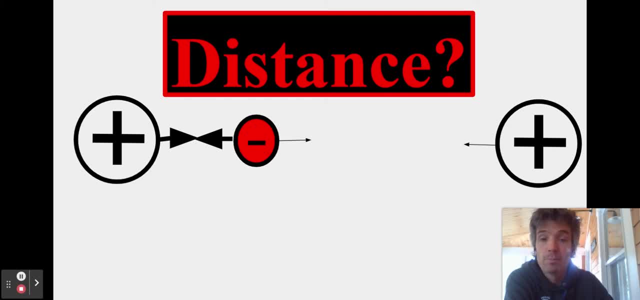 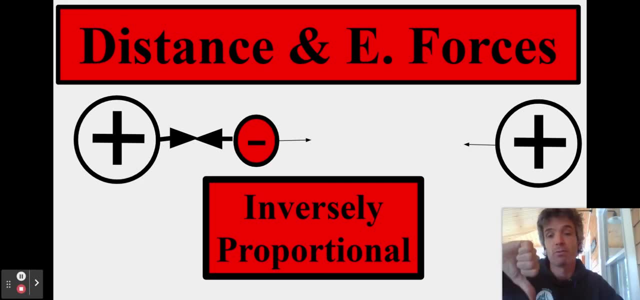 attractive force is going to increase. So what's the relationship with distance? Well, if I bring it closer, then it increases, and then it would raise. It would only increase, All right. So this is going to be inversely: The distance is going down and the electric force is going up. 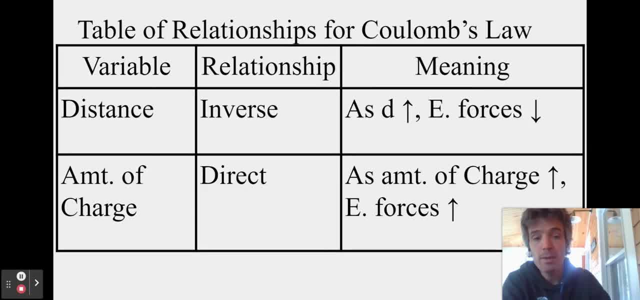 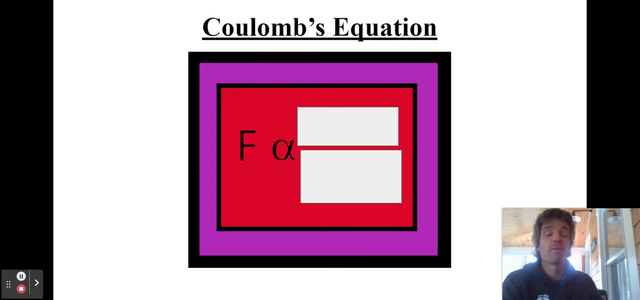 All right, So that's like an opposite trend. Here's a table showing you all the things Now in an equation, this force of attraction or of repulsion is proportional to two things. It's directly proportional to charge- therefore charge is going to be in the numerator. and it's inversely proportional to the distance, therefore the distance is in the denominator. 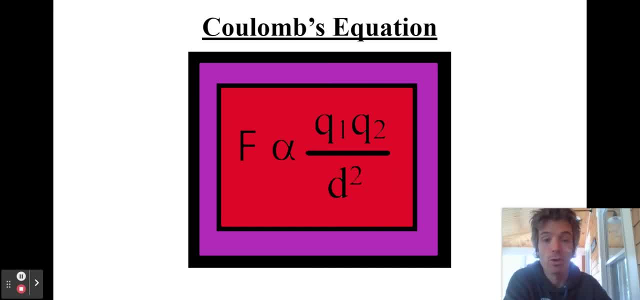 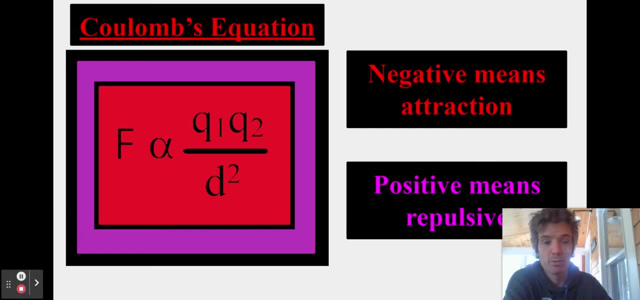 And the distance is squared. in this scenario, The Q1 and Q2 are the two different charges. Now I meant to. I should have added some shouldn't have this here. Anyways, for Coulomb's force, when you calculate it, a negative in this case would mean attraction and positive would mean repulsive. 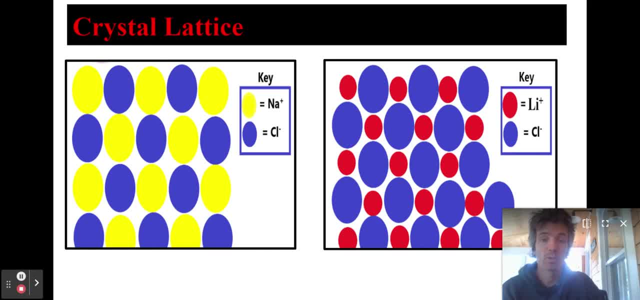 Now let's apply this to some crystals, two crystals being sodium and lithium. Now you can see, there's no difference. There's no difference in the charges of the respective ions, the cation and the anion. that both scenarios plus one and negative one. 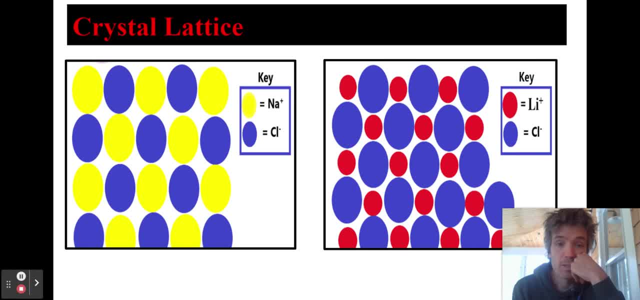 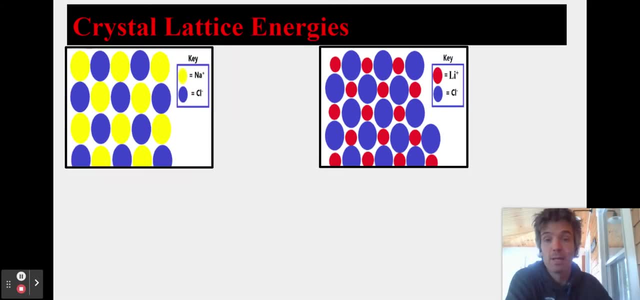 However, lithium's ions are significantly smaller than sodium's and you can see that that makes the distance go down. Therefore, the electrostatic force would increase. Now how does this apply to their lattice energies? That means it's probably going to make lithium chloride's crystal lattice stronger. 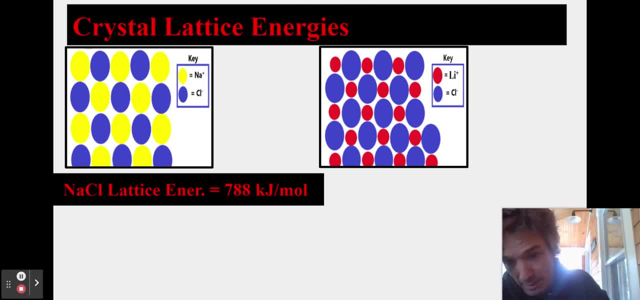 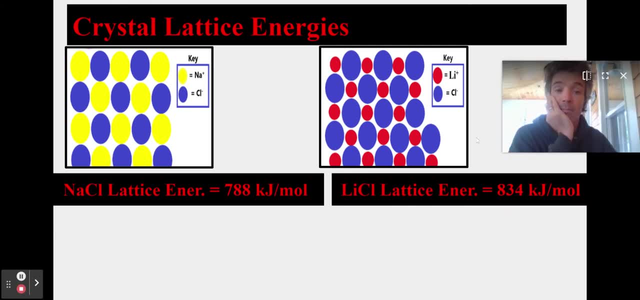 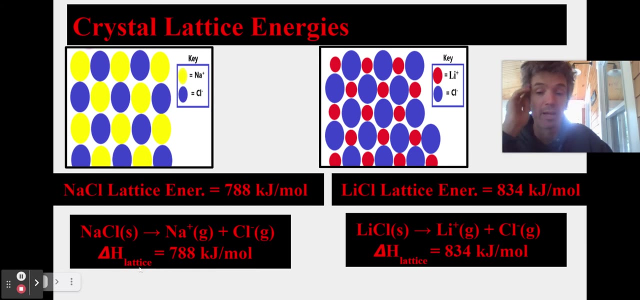 Here's sodium- how many sodium chloride's lattice energy. and there you can see this is lithium chloride's lattice. It's about 60 kilojoules per mole higher. And here's another way of writing it: You're going to delta H lattice, the change in enthalpy. all right, it's the same thing. 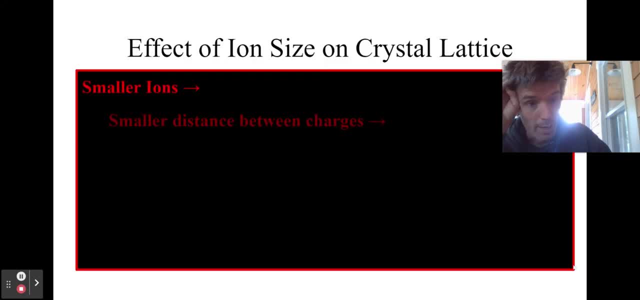 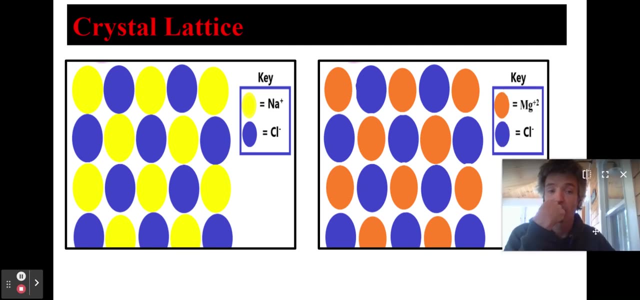 So the smaller the ion, the smaller the distance, the stronger. All right, Now let's look at a different crystal. This time we're comparing sodium to magnesium, and they're like next door to each other: Magnesium is 20.. 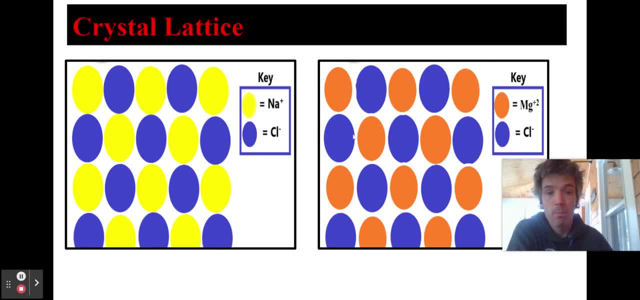 Magnesium is 12.. Sodium is 11 on the periodic table Now here sodium is a bit bigger than magnesium, about I think it's like 20 picometers bigger but it's. but it's got a magnesium's got a significantly larger charge, double the charge. 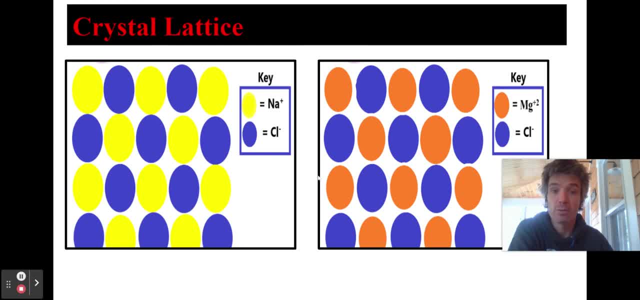 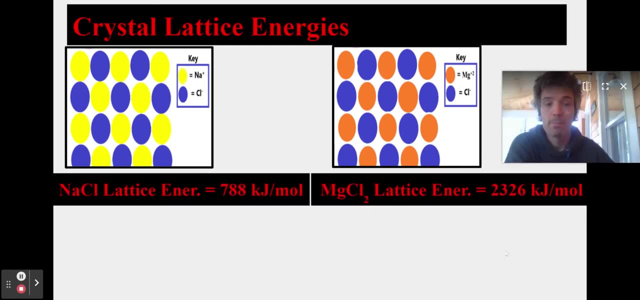 Therefore, you'd expect the lattice energy to be a lot greater over here than over there, because the bigger the charge, the more the attraction. Let's see if it, if it, plays out. As you can see, magnesium's is much, much higher. 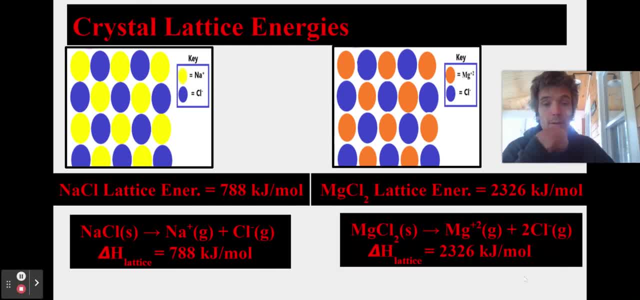 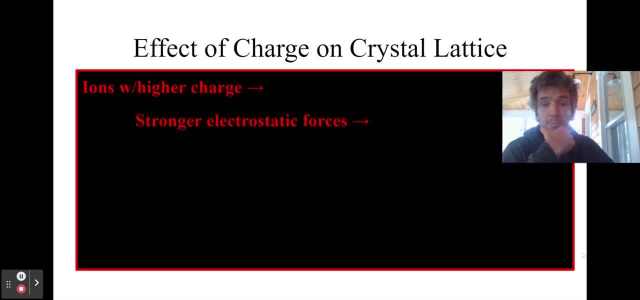 All right, It's almost triple the lattice energy. Here's the logic. Now, one thing: it says stronger lattice energy. It says stronger electrostatic forces. This is implying that they're going to be opposite and this electrostatic force is going to be attractive. 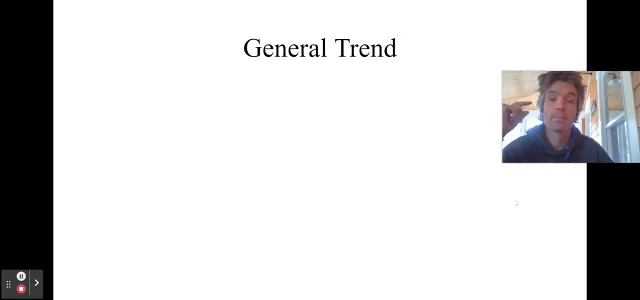 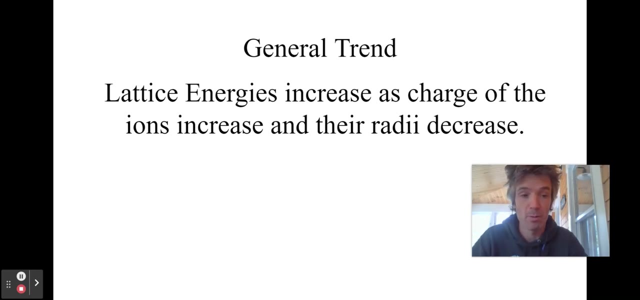 And the general trend here is: as ionic charge goes up, lattice energy goes up. As radius goes down, lattice energy goes up. All right, All right, I hope that's been helpful. All right, Have a good day and I'll let me know if I can help you out.